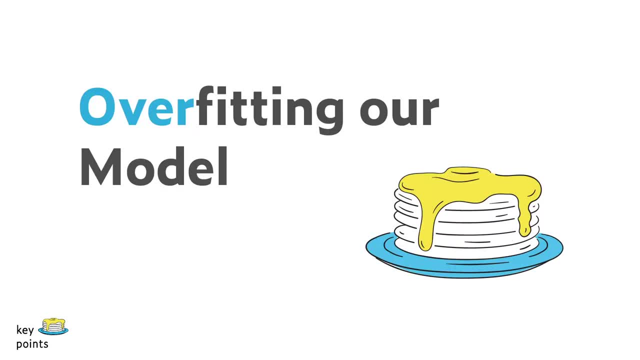 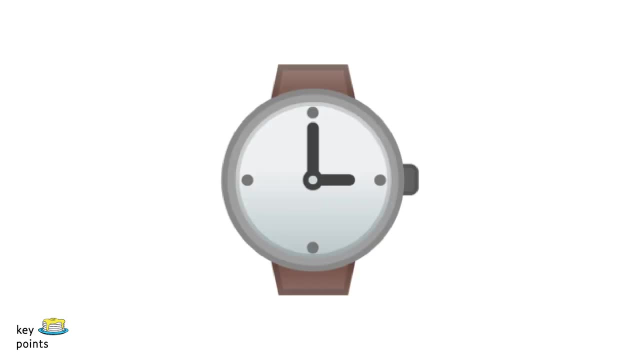 20 cups of sugar. Likewise, if we overfit our model, we might have splits like one grain of sugar, two grains of sugar, three grains of sugar, and so on and so forth. Counting out grains of sugar is going to take far too much time And will we even be able to perceive. 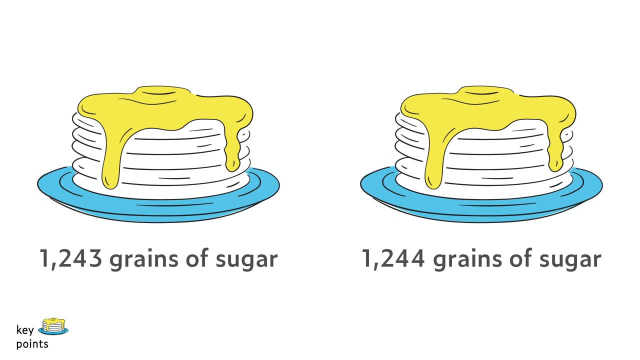 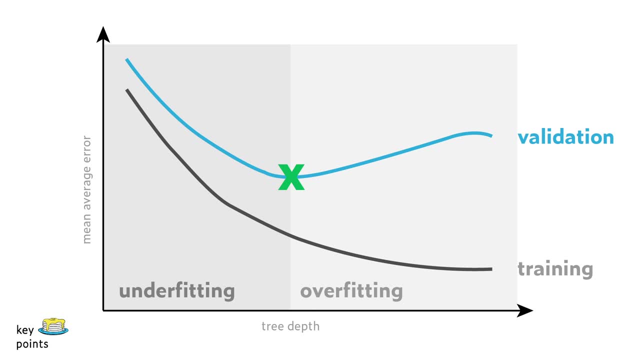 the difference between a recipe made with 1,000 and 243 grains of sugar and one made with 1,244 grains? Probably not. What we really want to do is strike a balance between overfitting and underfitting. So when we're trying to find the balance between overfitting and underfitting, one of the things 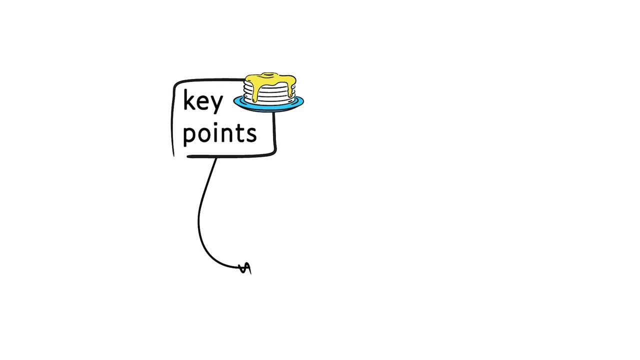 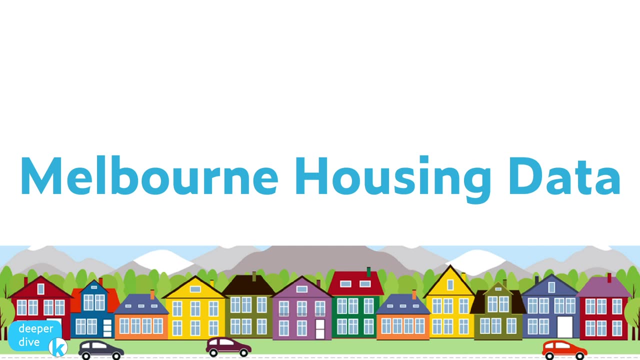 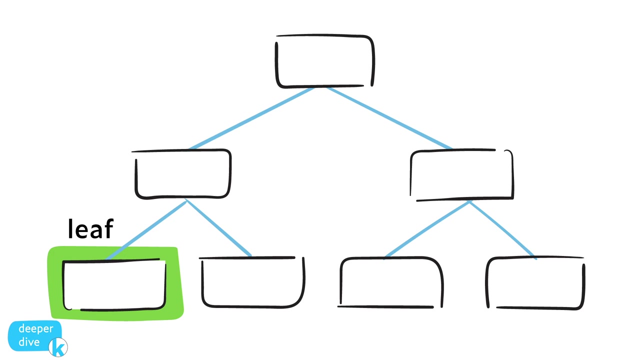 we can do is modify our model's parameters, And while there are usually a good number of parameters that we can modify for our purposes, we're going to focus on modifying the maximum number of leaf nodes in our decision tree model, regression model. So let's think about this for a second. If we allow our decision tree to create, 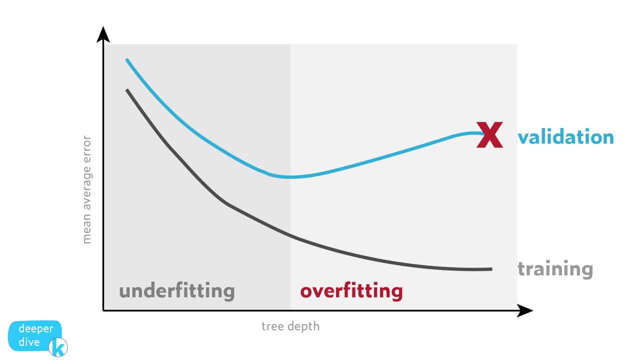 thousands of leaf nodes, we could hypothetically end up with a tree that has a leaf for every price within our training data set. This would be an example of overfitting, because the model would fit our data almost perfectly, making it challenging to generalize to a new data set. 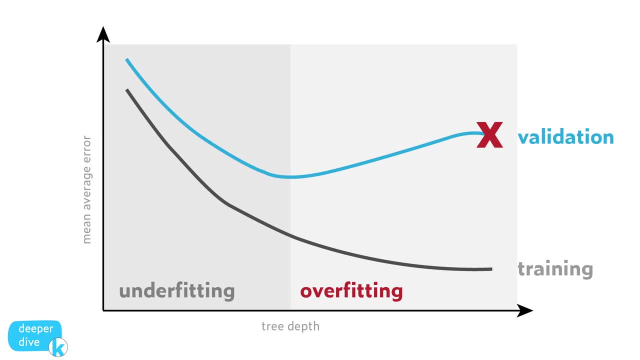 When we overfit, the model doesn't perform as well because the validation data doesn't always look like the training data. As the tree gets more complex, we see our validation error rise and what's happening is that it's become easier for the tree just to memorize all of the specifics. 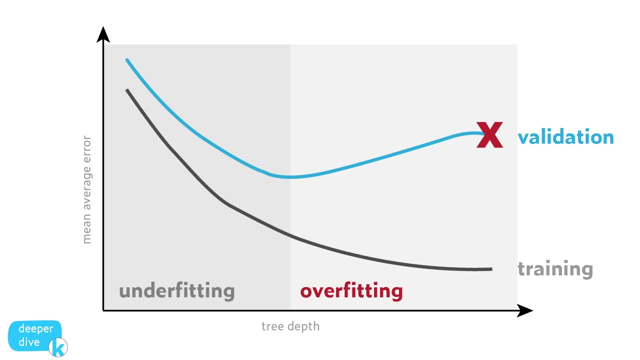 in the training set than actually learning the general rules. Likewise, if we only allow our decision tree to have a small number of leaf nodes, let's say four, kind of like we saw in our earlier lesson, then we would have a model that has been underfit Any predictions we try to make about. 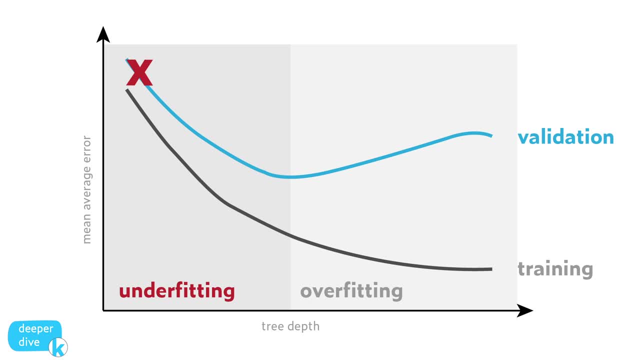 housing prices would be so general as to be next to useless. One way to think about this trade-off is that when we start with just a couple of leaves, we're underfitting our model. As we add more leaves, we're moving in closer to the tree. So if we add more leaves, we're moving in closer to the tree. 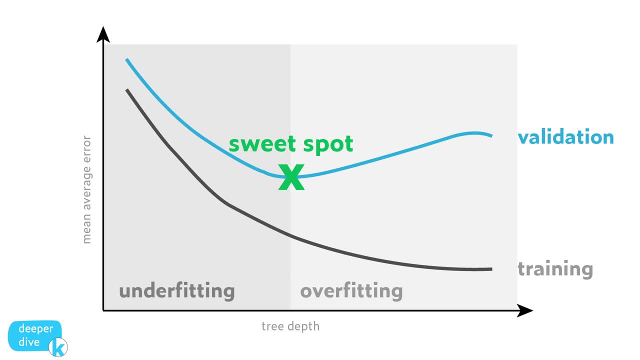 So if we add more leaves, we're moving in closer to the tree. So if we add more leaves, we're moving in closer to the tree- a sweet spot where our model is going to be pretty good at predicting housing prices on data it's. 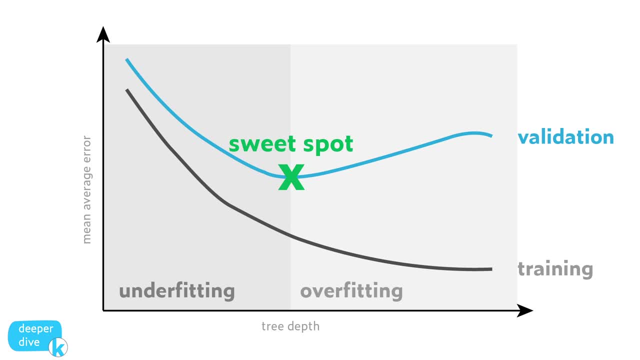 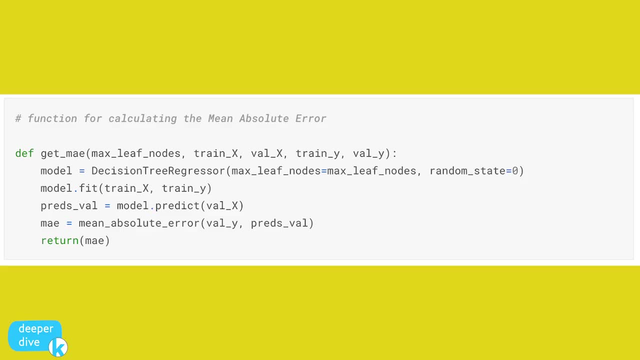 never seen before. but we can actually have too much of a good thing. If we keep adding leaves past our sweet spot, we'll likely end up overfitting our model. So in the lesson we saw that there was a function written for us to calculate the mean absolute error relative to the number of leaves.